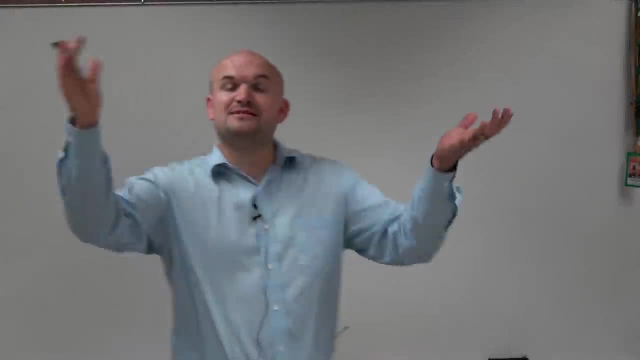 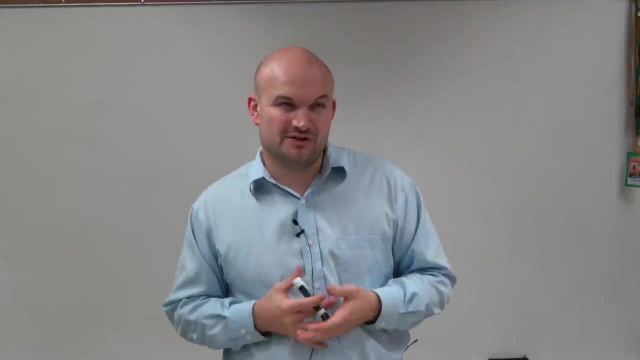 Welcome, ladies and gentlemen. So what I like to do is show you how to determine if a function is even or odd or neither. Now there's kind of two different ways we can do this. We can do this one by looking at the graph, as well as two looking at this algebraically. So I 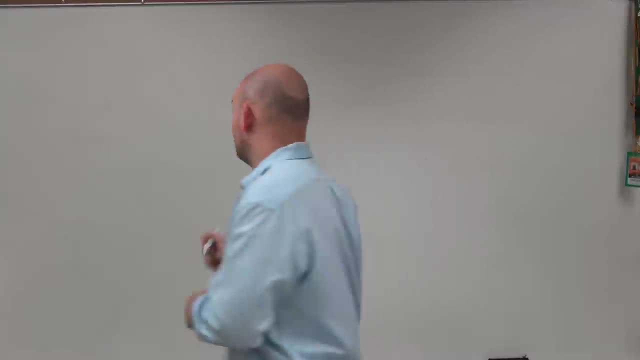 think the best way to kind of start off this is by looking at it graphically. So when we have even functions, even functions graphically are symmetrical about the y-axis. So let me just kind of give you an example here, This graph: you can see that the y-axis perfectly. 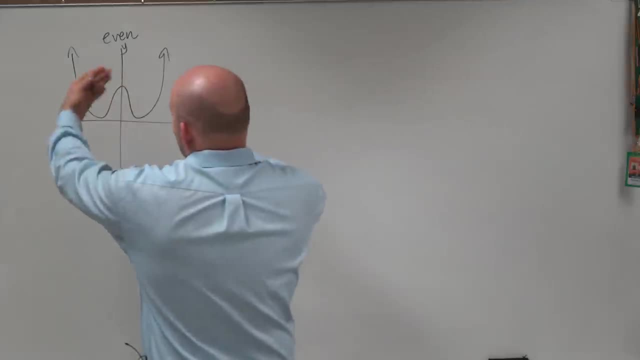 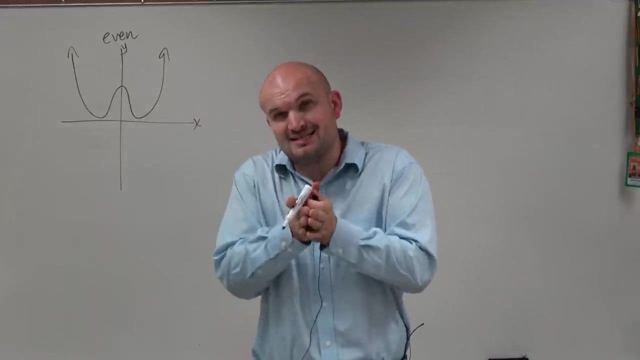 splits up the graph. It's the exact same on the left and the right side. Again, I apologize for my shading, but you can see that this is definitely going to be an even function where the y-axis is your line of symmetry. So even functions are symmetrical about the y-axis. 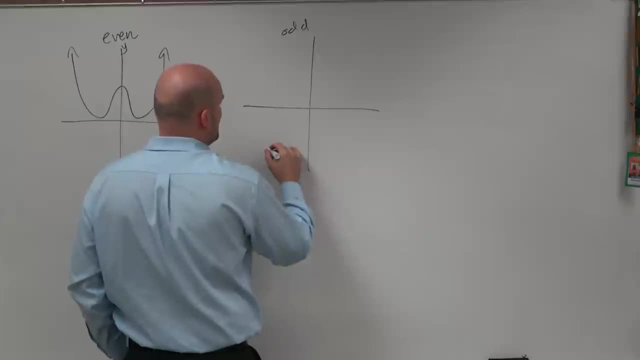 Odd functions are going to be ones that are symmetrical about the origin And basically, another way to think about symmetrical about the origin is if you reflect them about the y-axis as well as reflect them about the x-axis, you're going to get the exact. 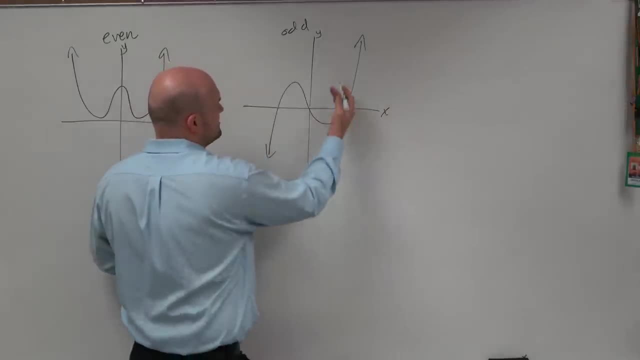 same graph. Now again, I'm not perfect with this, but again these points: if you were to reflect this about the y-axis and then reflect it one more time about the x-axis, you should have the exact same graph, And then obviously neither is going to be functions that do not have any symmetry. 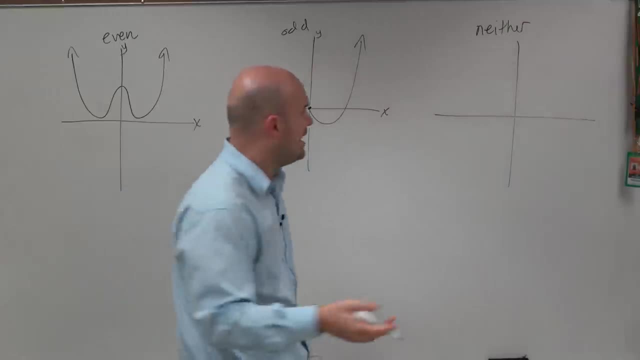 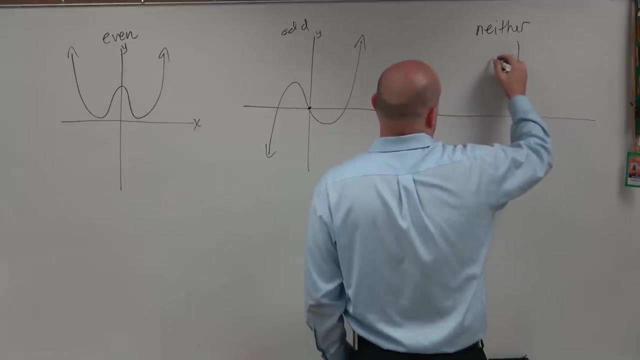 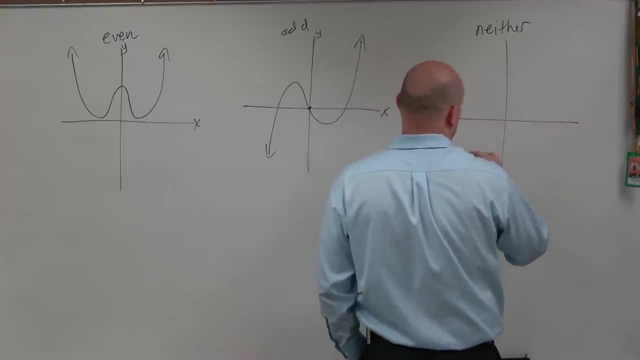 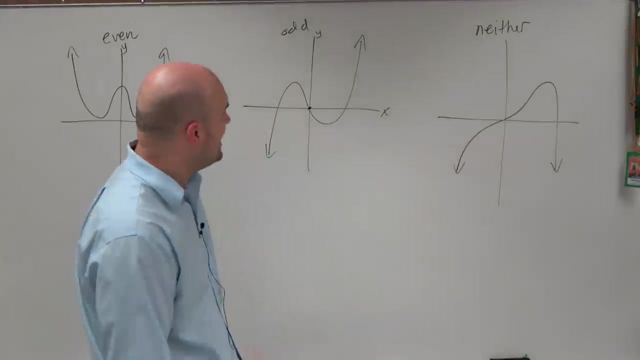 get some kind of function that we know of. There we go. That graph has no symmetry across the x or the y-axis, So that is neither Now the main important thing. the way to find this. algebraic is usually where students get a little mixed up. 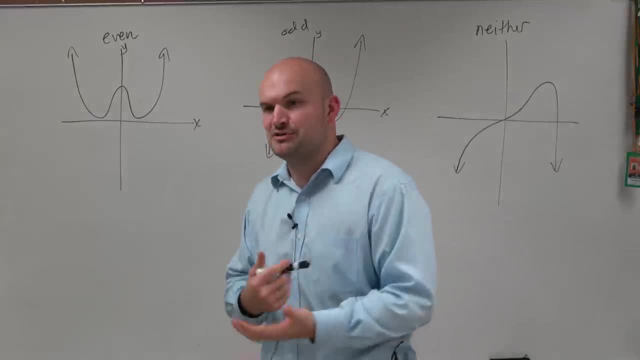 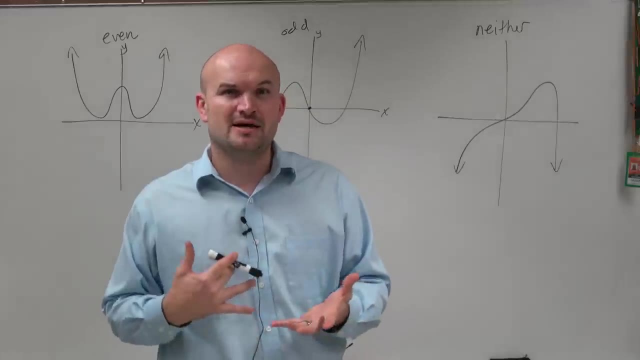 By the graph. it's kind of simple because we've been talking about symmetry a lot in the course as well as in previous courses, So identifying symmetry is not so bad. But it's usually when we get to the algebra that we start making kind of some. we start having some issues. 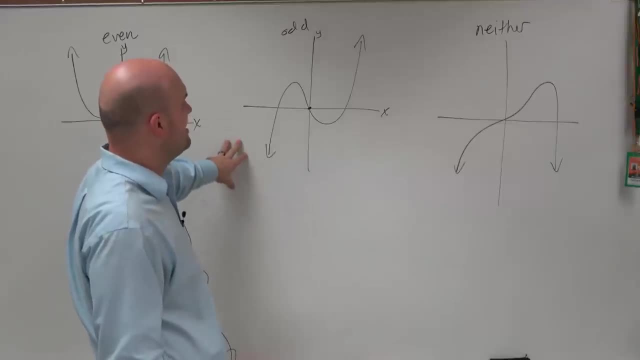 So what I like to do is always refer back to the graphs and kind of make some sense as far as how can we use the graph to help us understand algebraically what it means if a function is even odd or neither? So the best way I like to do that is just picking a point. 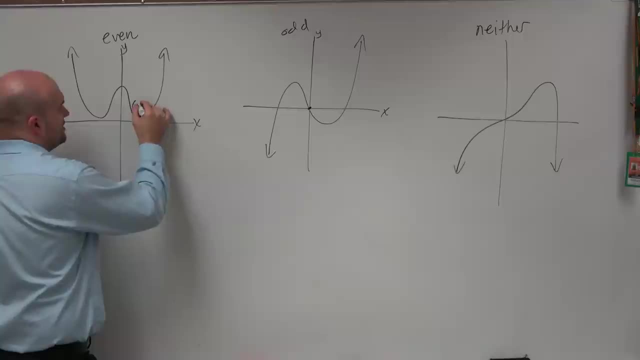 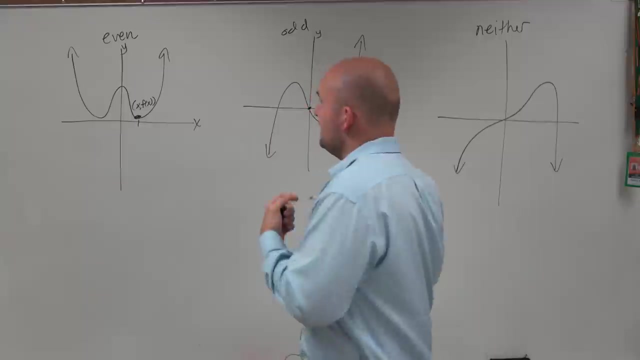 So let's pick some random point here, And this random point is going to have the coordinates x, comma, f of x. x is the input, f of x is the output, just like an x and y coordinate. Now, if I was about to take this function, 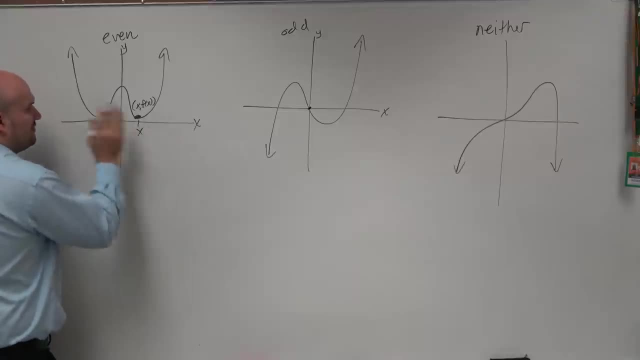 if I was going to take this point, let's say so. this is x. Let's reflect this point. Therefore, that's going to be negative x. So what happens is when I have negative x, I'm still going to get f of x back out. 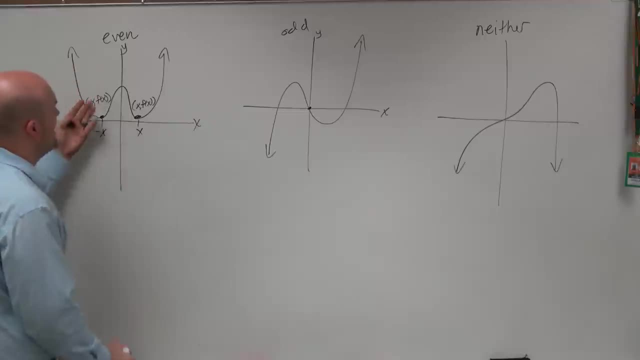 And that's really the essential of the even function, Since they're symmetrical about the y-axis. if you have x over here and negative x here, they have the same distance away. their heights are always going to be exactly the same And it doesn't matter what two points you pick. 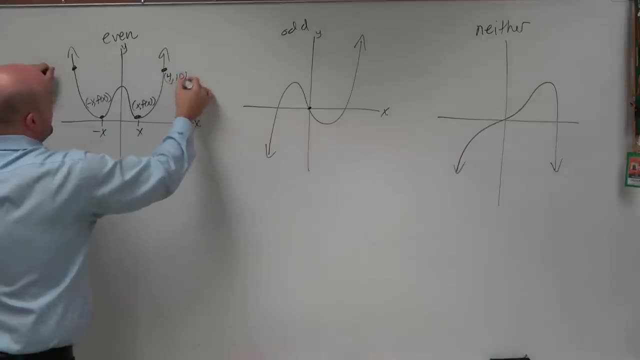 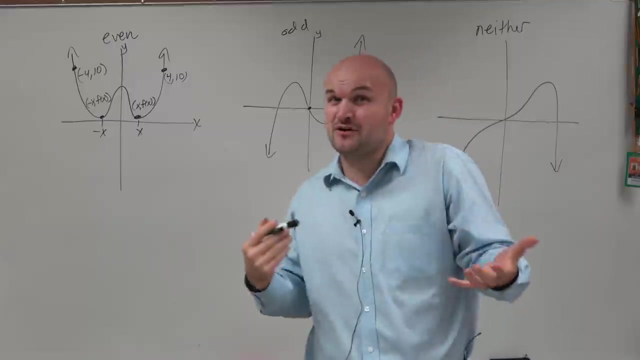 If this is like 4, 10,, well then this point would be negative: 4.. 10 because of the symmetry. So the way to test that for any function, especially one that you have no idea what the function is, is basically to plug in f of negative x. 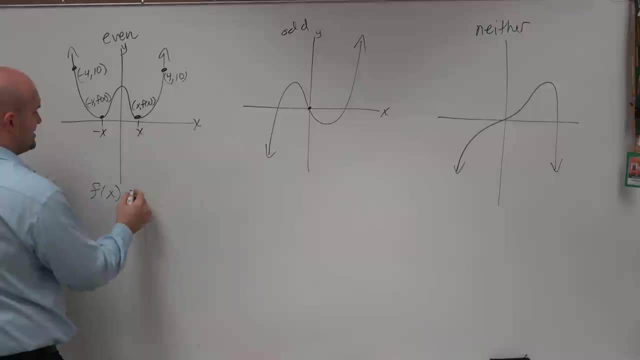 So we know that if we plug in f of x or if we plug in x, we're going to get our function f of x. I mean, f of x is equal to f of x. Whatever value you plug in for x, you're going to get it. 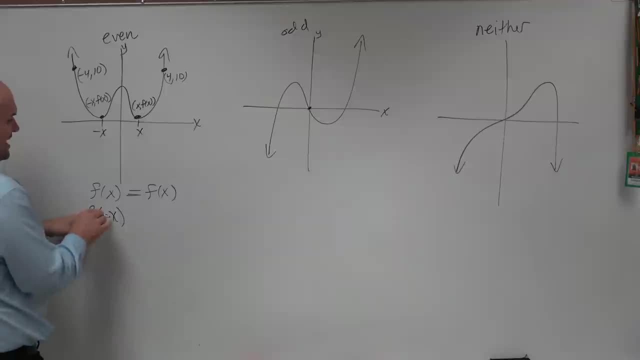 The definition of an even function algebraically is: if I plug in negative x, I am also going to get f of x, And again, that makes sense. Remember, I plug in for x. I should have the exact same output if it's positive. 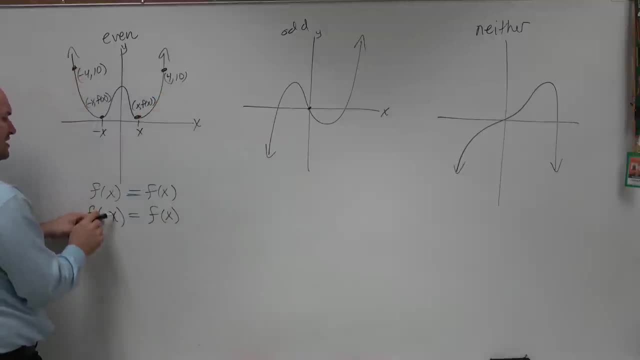 or if it's negative. So to test a function, you're going to plug in negative x, evaluate the function and simplify, And if you get the original function, then your function is even For odd, it's a little bit different. 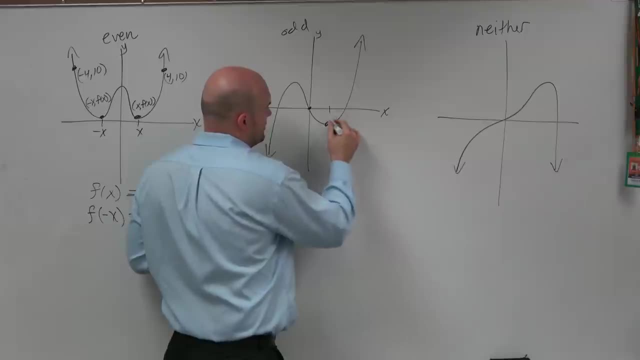 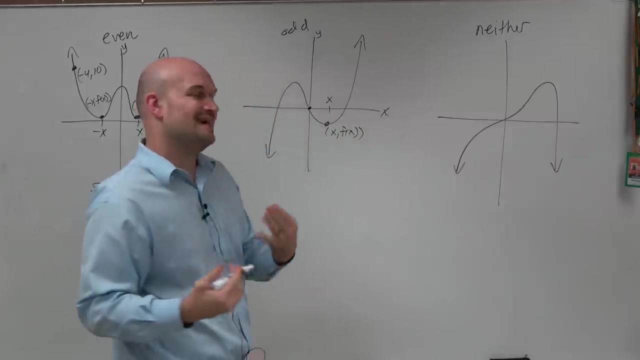 Here is my function. Here's my x, So here's x. So this coordinate is x, comma f of x. So remember it's reflective about the origin, which is the x and the y-axis. So if I reflected about the y-axis, 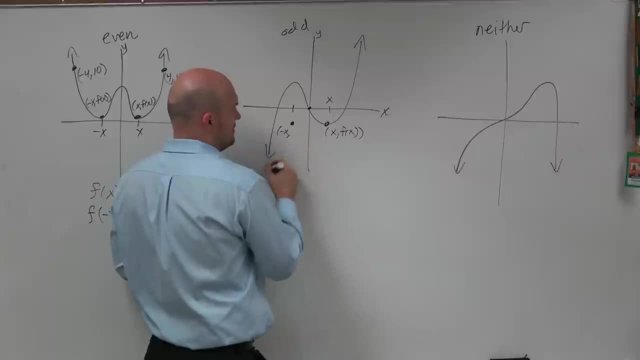 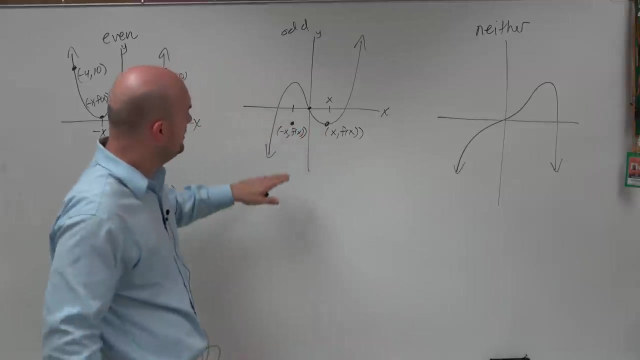 this point is right here- which would now be negative x, And it's still f of x. Now again, that f of x is negative is a negative value, But the important thing I want you to understand is it's still the same answer. 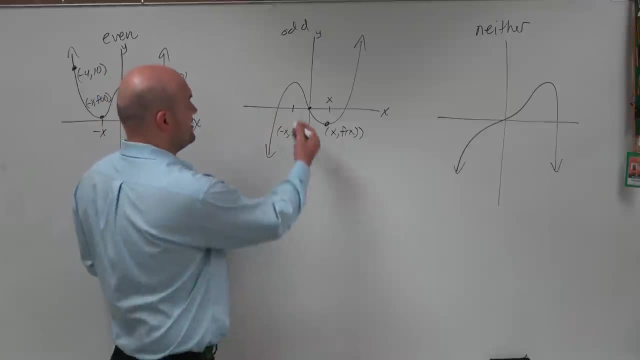 Maybe I should. yeah, Then if I reflected about the y-axis over here, I still have negative x, but now I have the opposite of this value, which would now be a positive. Oh, that can be kind of confusing. Let's look at this. 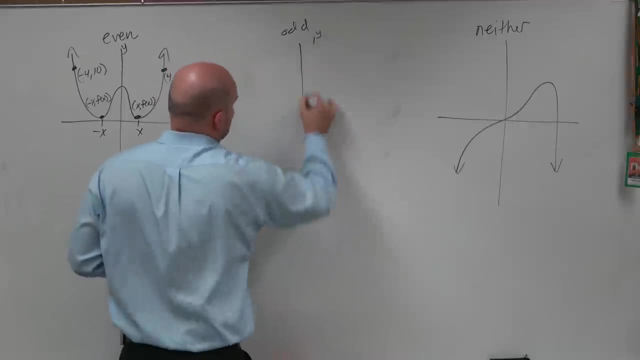 Let's look at a different graph just so I don't overly confuse some people, because it doesn't really make sense. I mean it doesn't really matter what it works like, But let's just deal with kind of positives. So let's look at this is an odd function again. 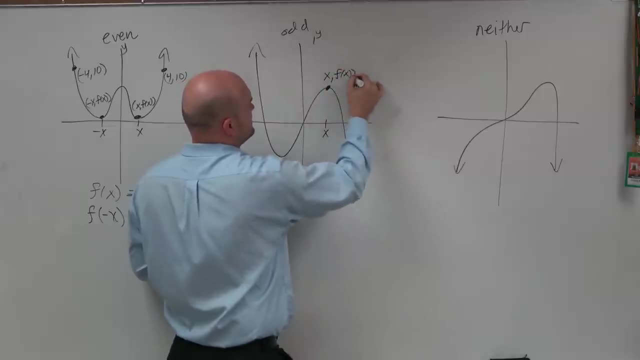 So here's my value x. Here's x comma f of x, And at least this time f of x is positive. It is positive Now again, when I reflected about the y-axis, I'm now dealing with negative x, but still I. 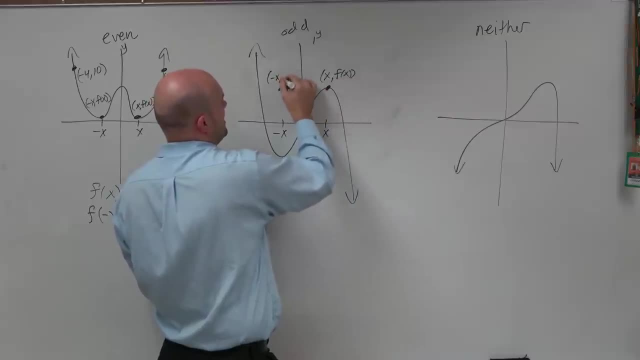 have the same value of f of x. So this is negative x comma f of x. So now, if I reflect this about the x-axis, I'm still at the same coordinate point- negative x- but now I'm at the opposite value of f of x. 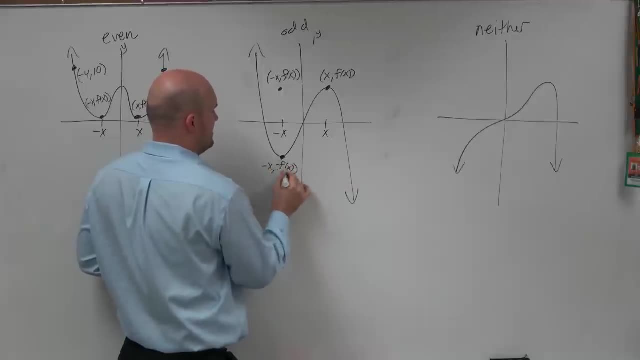 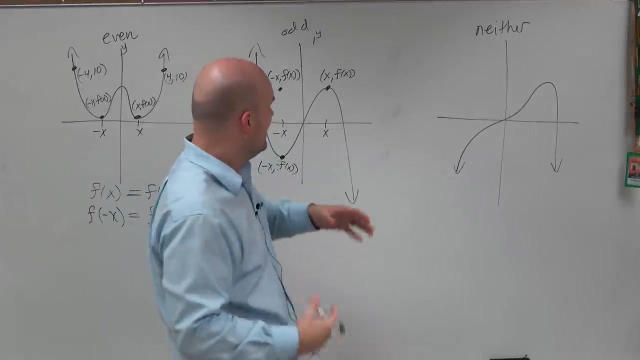 which is opposite f of x. Now again, my previous example was perfectly fine. I just You've got to be careful with understanding if it's positive, negative and opposite. I just didn't want people to be confused with being negative and opposite. 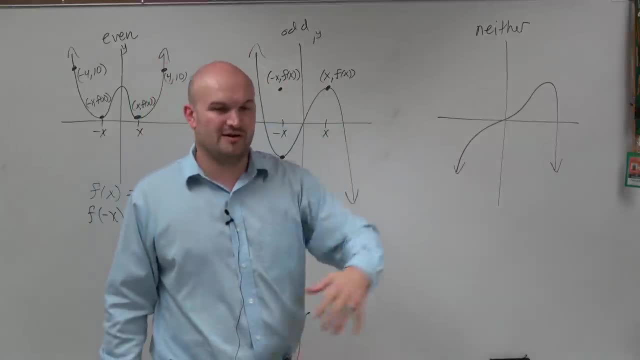 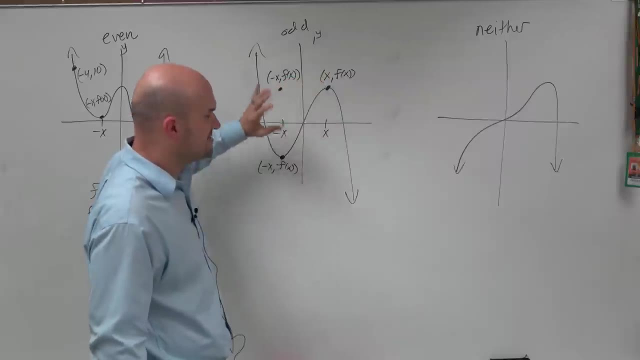 So the previous example would have worked As an introductory video. I just wanted to keep things positive and negative as they are. But you've got to be careful because, remember, these negatives are representing the opposite value. So the definition here of an odd function is: if I have f of x, 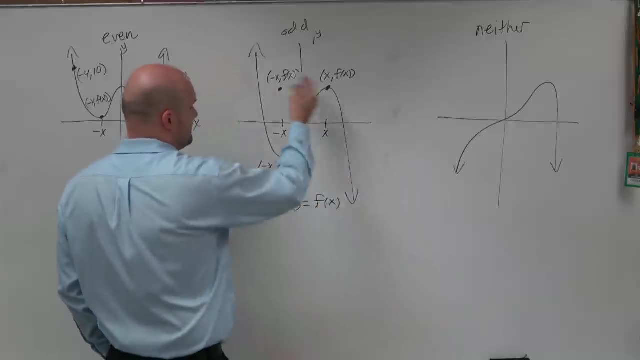 plug in f of x, I'm getting f of x. Well, if this function is odd, that means, if this is an odd function when I plug in f of negative x, I shouldn't get up here, right? If I get the same value then it'd be even.